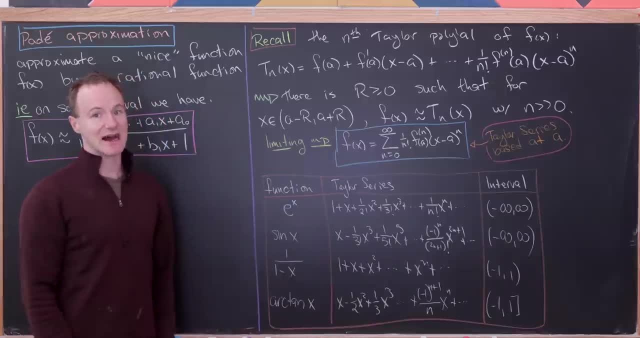 our original function, and that is if we have a nice enough original function. Now here are some, like well-known common Taylor series, where we base them at a, And you can see that we can simply truncate these to get Taylor polynomials of whatever degree that you want. 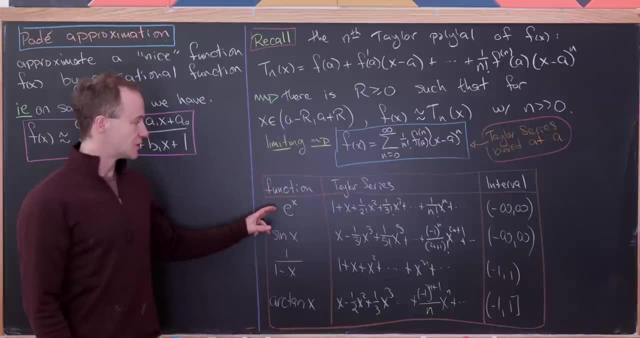 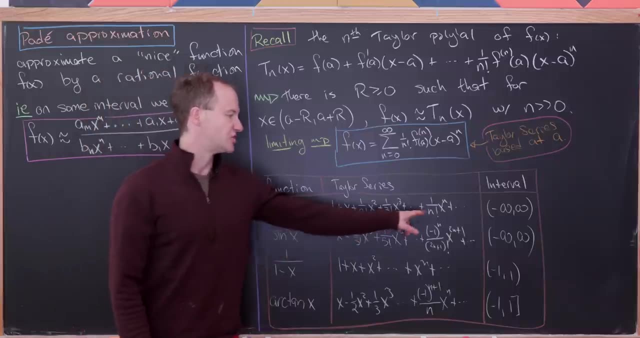 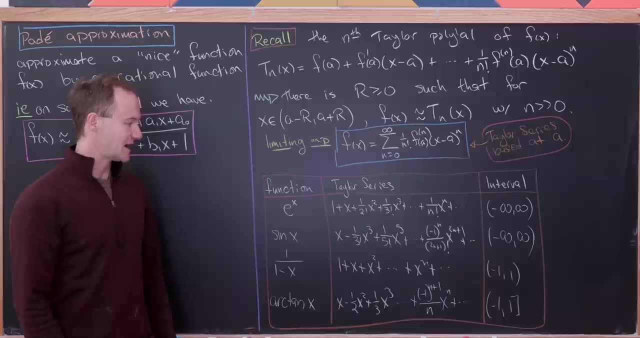 And here we're taking a to be equal to zero, if I didn't say that. So for e to the x, we get this Taylor series which is one plus x plus one over two factorial x squared. The general term is one over n factorial x to the n. For sine of x, we have x minus one over three factorial x cubed plus. 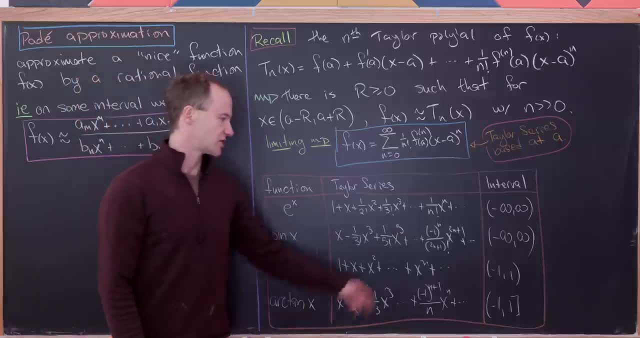 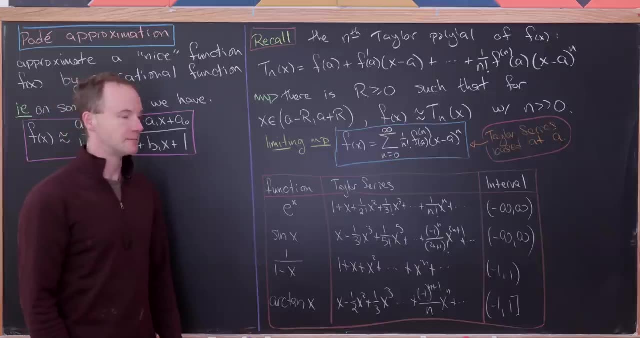 one over five. factorial x to the fifth is minus 1 to the n over 2n plus 1, factorial times x to the 2n plus 1.. And the intervals for these first two are simply all real numbers, so we get convergence everywhere. Then 1 over 1 minus x. 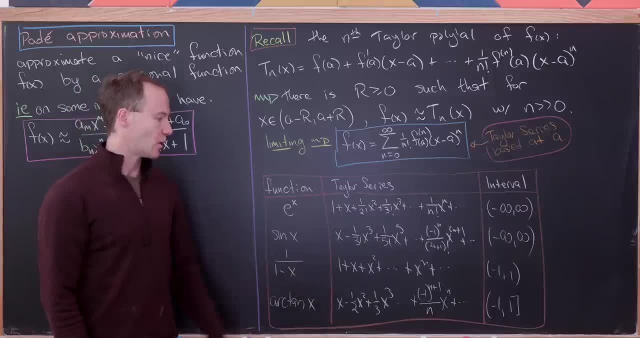 well, that's just a standard geometric series. So we've got 1 plus x plus x squared. The general term is x to the n, The unit interval, the open unit interval, that is, is our interval of convergence. Next up for the inverse tangent, we have x minus a half x squared, plus a third x cubed. 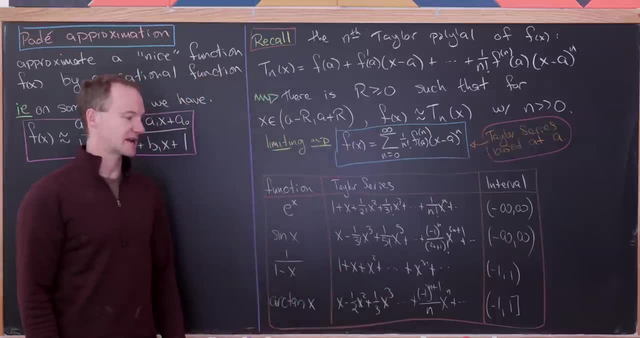 The general term is minus 1 to the n, plus 1 over n, x to the n, And here we get the unit interval that's open on the left and closed on the right. Okay, so now that we've recalled this polynomial method of approximation, let's jump into our rational function method of approximation. 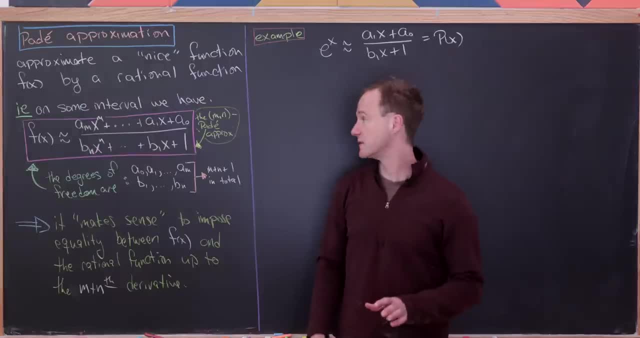 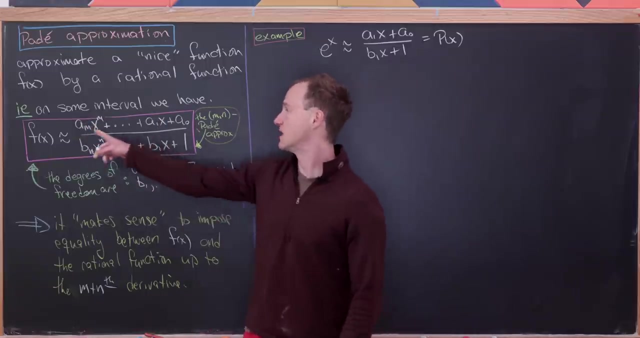 So this type of approximation is called a Poisson approximation. And just to reiterate, we want to approximate our nice function by some sort of rational function, That is, on some interval we should have. f of x is approximately equal to on the numerator we. 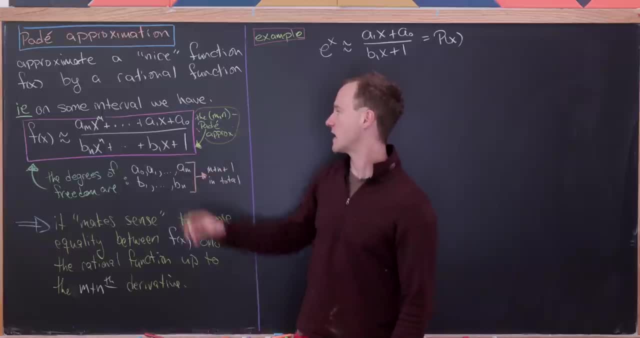 have a sub n x to the n added all the way down a1x plus a0.. In the denominator we have b sub n x to the n added all the way down b1x plus 1.. So we can always multiply the numerator by the denominator. So we have b sub n x to the n added all the way down b1x plus 1.. 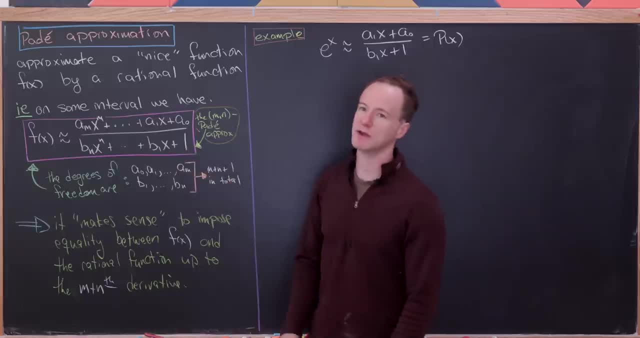 So we have b sub n, x to the n, added all the way down b1x plus 1.. So we can always multiply the numerator and the denominator by something to turn this number into a 1.. We could really put a 1 anywhere we wanted, but we might as well put it there And this is called the m comma n. 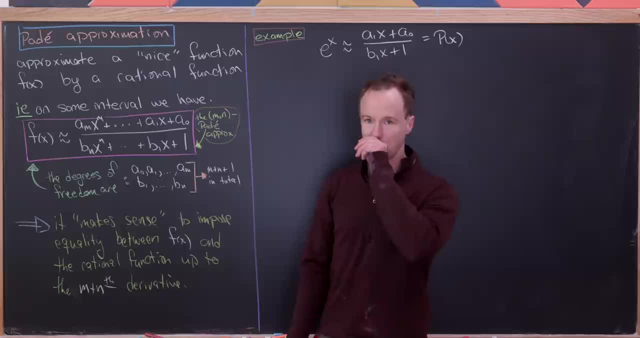 pod a approximate. Now I'd like to point out that inside of this rational function there are m plus n plus 1 total degrees of freedom, And those are those coefficients that we have. But m plus n plus 1 gives us the ability to. 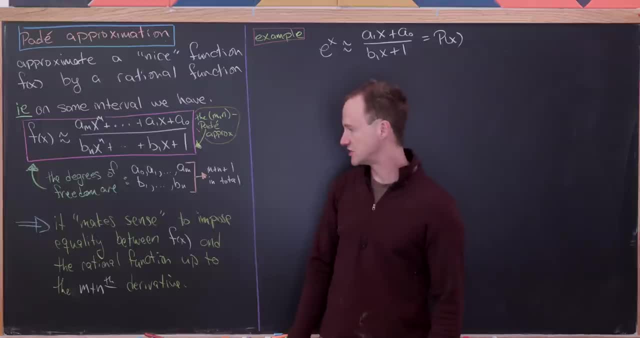 to impose m plus n plus 1 equations, And the way that makes sense to do that is to impose equality between f of x and the rational function up to the m plus nth derivative. Now, why the m plus nth derivative? Well, that's because we're going to impose it for the zeroth derivative. 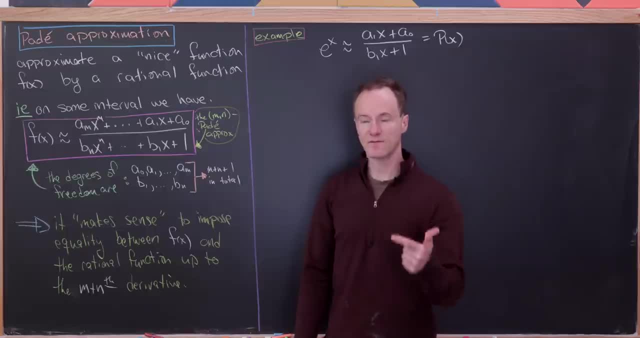 That is just the function value, Then the first, second, third, fourth, all the way up to the m plus nth, So that'll be m plus nth, And then we're going to impose equality between f of x and the m plus n plus 1 total, maybe things that we're setting equal to each other, total equations. 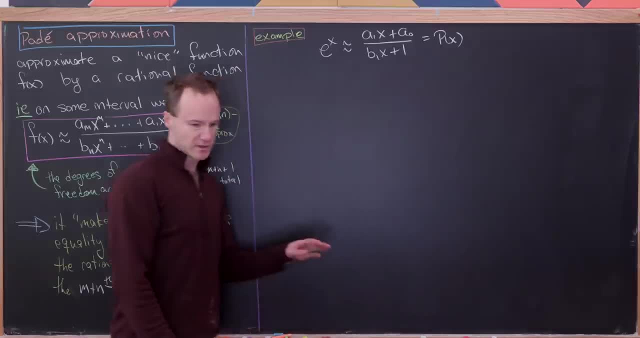 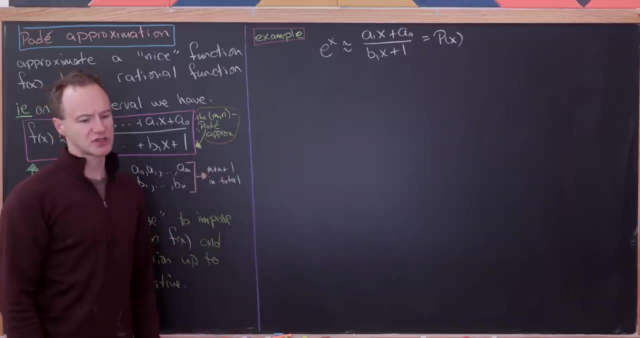 And these are like our unknowns. So let's do our first example. We'll look for an approximation of e to the x, where we have a quotient of linear polynomials, And I'll call this p of x. That's the rational function. Okay, so we've got three degrees of freedom. So that means we should have: 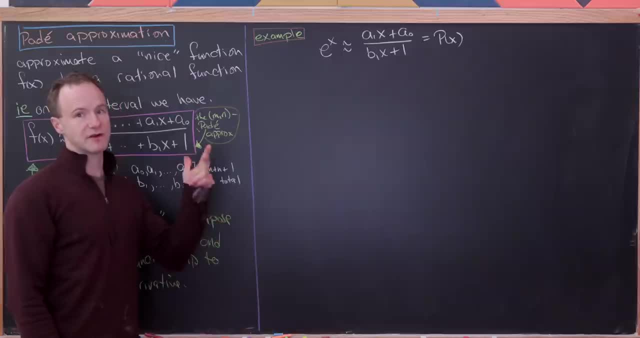 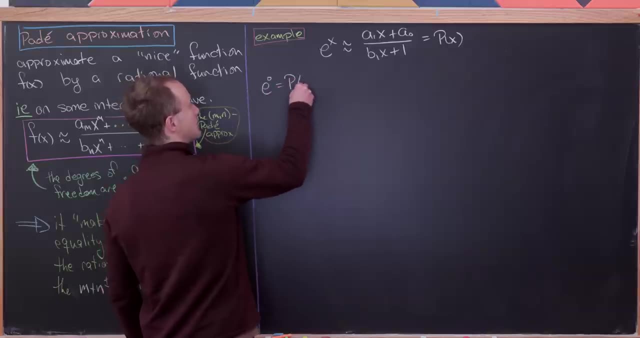 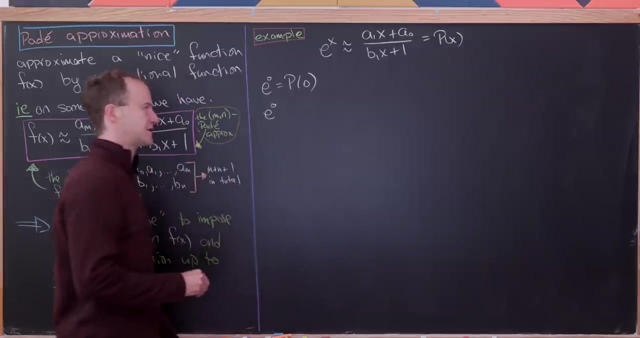 equality of of the functions, their first derivatives and their second derivatives. So in other words, we need e to the zero to be equal to p of zero. And then we need equality of first derivatives. Well, the derivative of e to the x is simply e to the x. So that's e to the zero, again equal to p prime of. 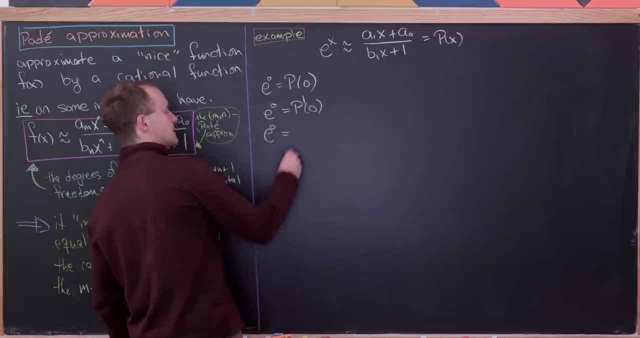 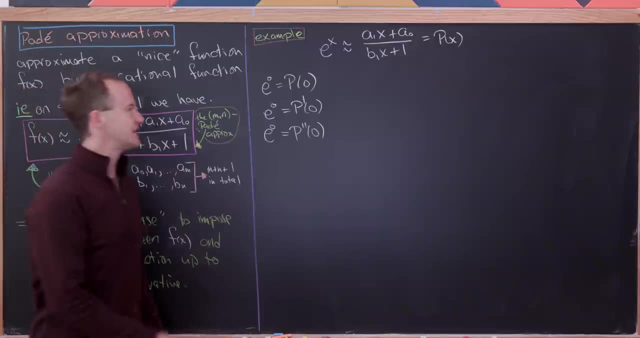 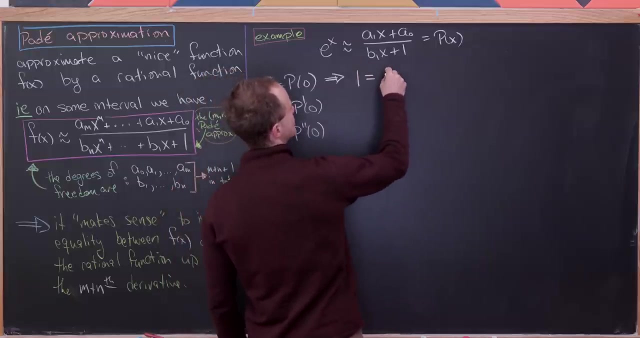 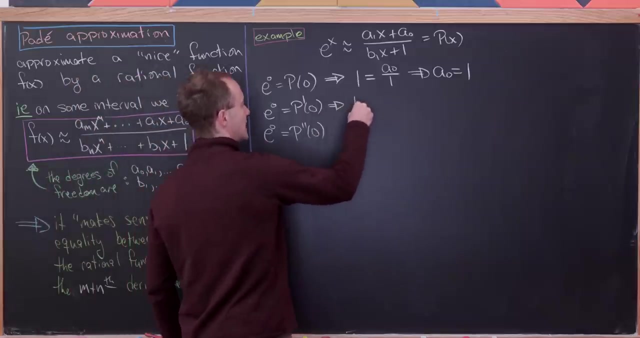 zero, And then the second derivative: well, that's just going to be e to the zero again, and p double prime of zero. So those are our three equations. So let's see what we get out of this. So e to the zero is one, And then p of zero is equal to. let's see a zero over one, Oh, but that means that a zero is equal to one, Okay, well, now let's look at this p prime of zero thing. Well, again, e to the zero is one, And then, if we take the derivative here, we'll get a. 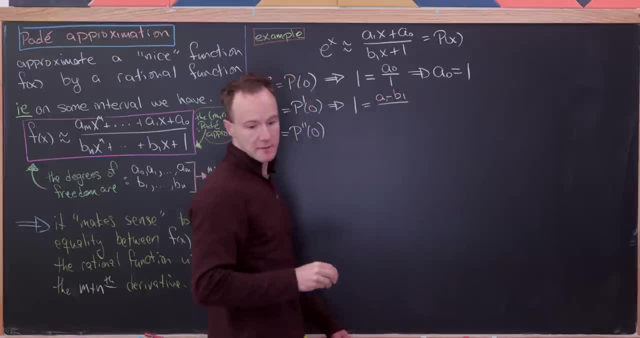 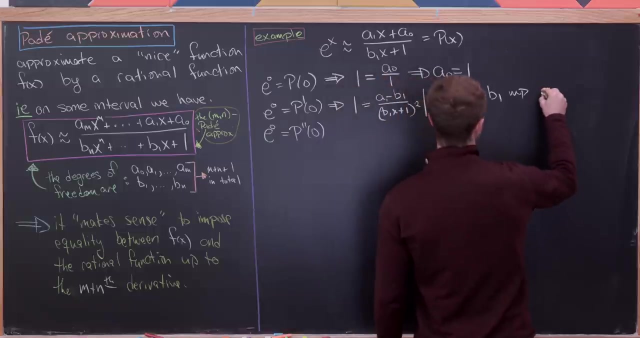 one minus b one over b one, x plus one quantity squared, then we need to evaluate that at x equals zero. So I just took the derivative. we have to use the quotient rule, obviously. But if we set x equal to zero, here we'll get a one minus b one. But then let's maybe put this all together: Here we'll have a one minus b one is equal to one. 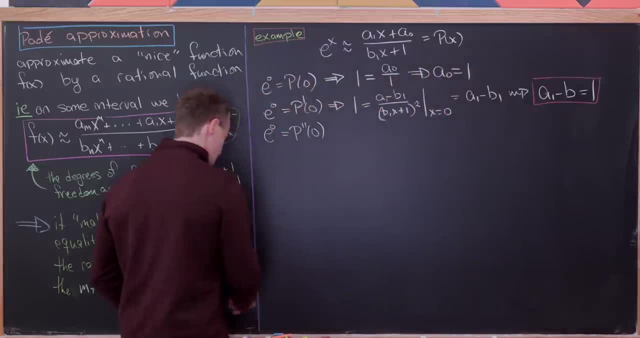 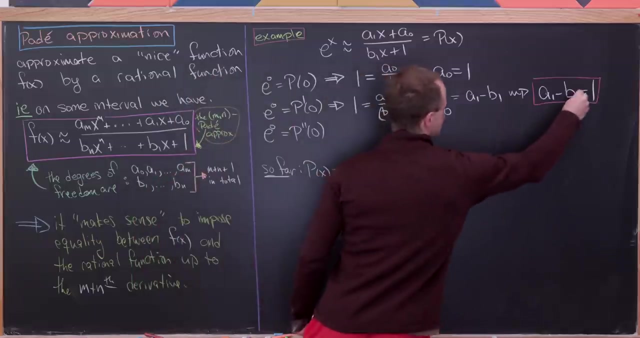 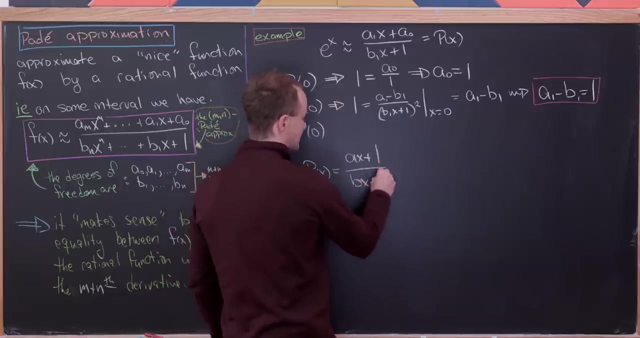 Okay, nice, But now let's maybe take a midpoint summary here. So so far, before we impose this third condition we have: p of x is equal to well, I'll just call this ax plus one over bx plus one, because we've already fixed a, not at one. And then here I'm renaming. 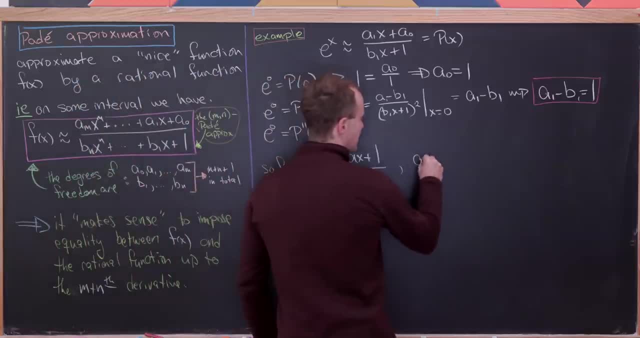 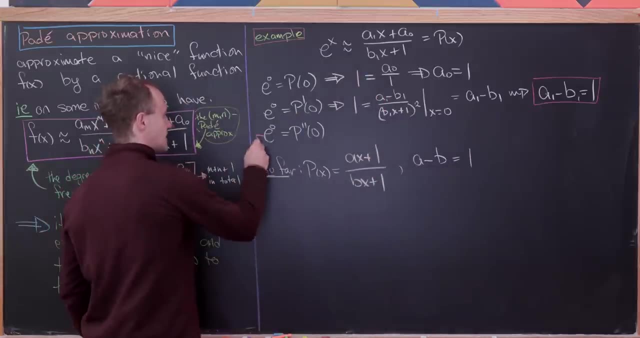 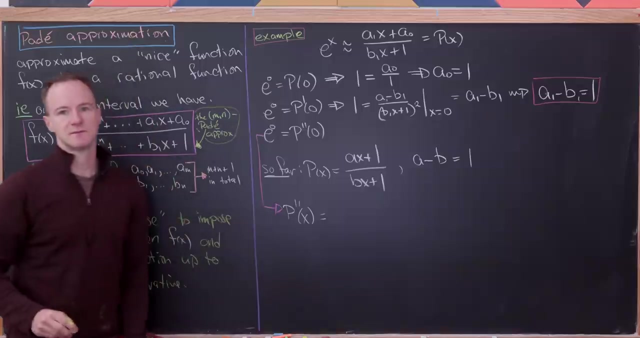 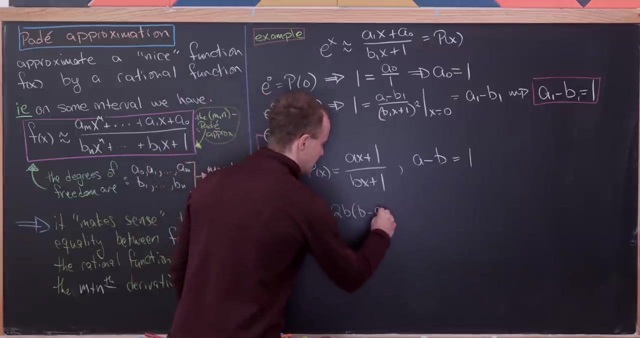 a one and b one just to a and b. And then those satisfy this: a minus b equals one. And now let's impose this second derivative condition. So that means we need to take the second derivative of p of x. Well, again, that's just by using the quotient rule a couple of times. Here we'll get two b times b minus a, all over bx plus one quantity squared. 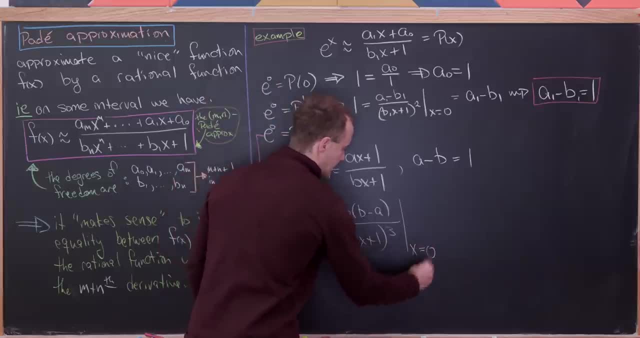 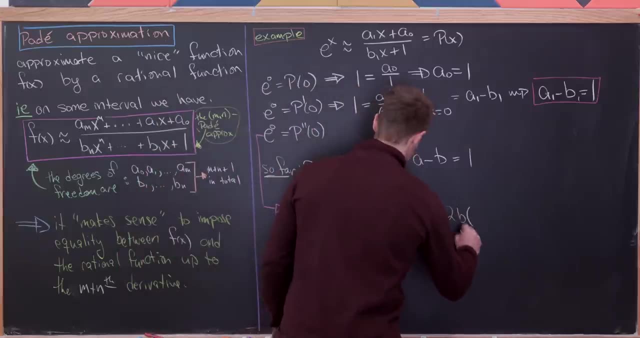 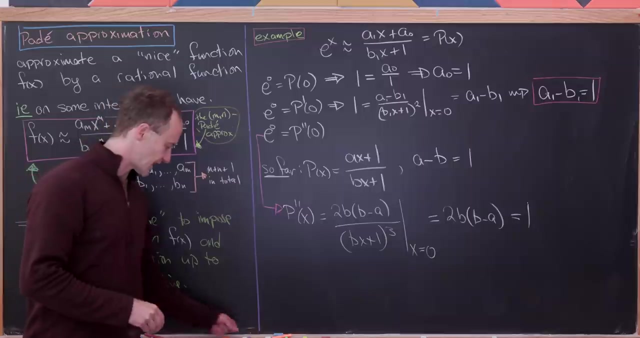 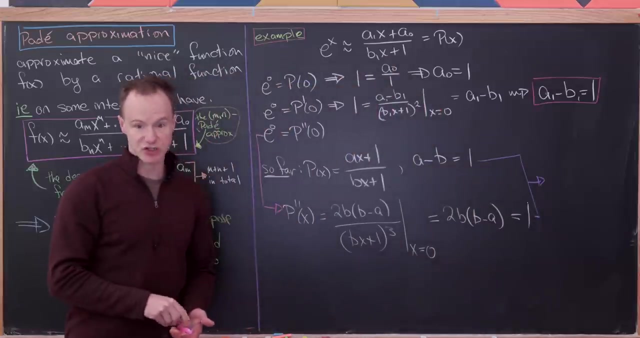 cubed. But now applying our condition that we need this at x equals zero. that's going to simplify down to two b times b minus a, and then we need that to be equal to one. So check it out. Now we've got two equations and two unknowns. So those are two equations and obviously the two unknowns are a and b. But observe, if a minus b is equal to one. 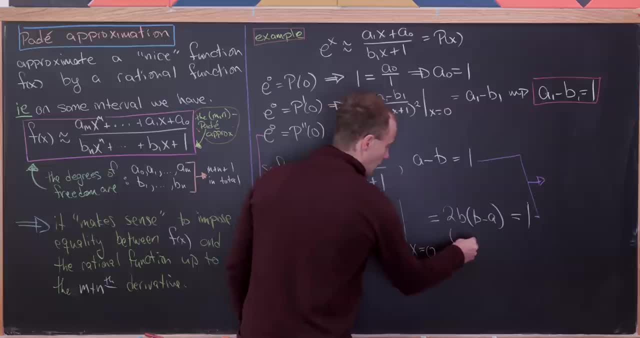 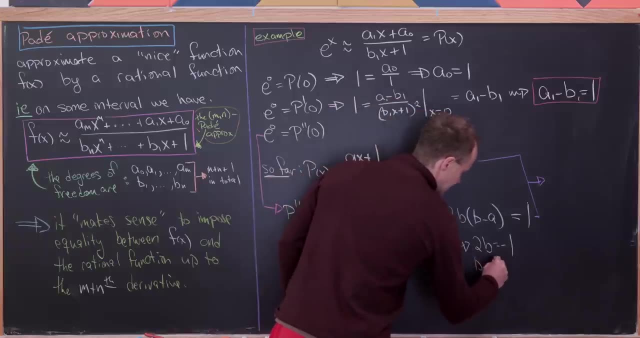 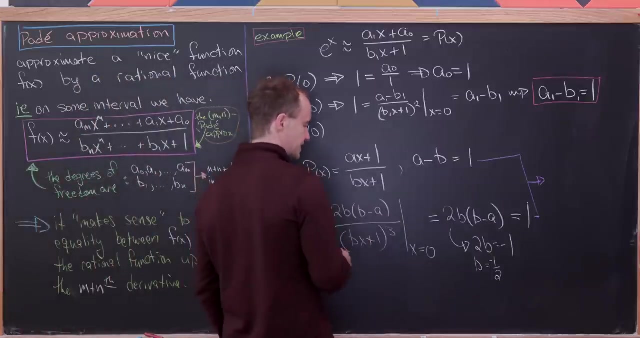 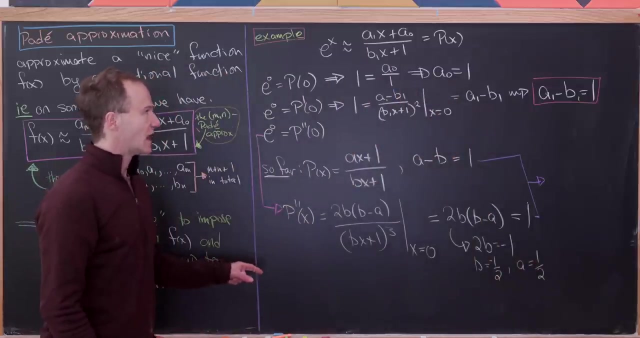 that means that b minus a is equal to negative one. Oh, but that means that two b is equal to negative one, Just moving the minus sign over, meaning that b is equal to minus one half. But then if b is equal to minus one half, plugged into this first equation we'll get: a is equal to one half. So that really turns our function into the following: So we have p of x. 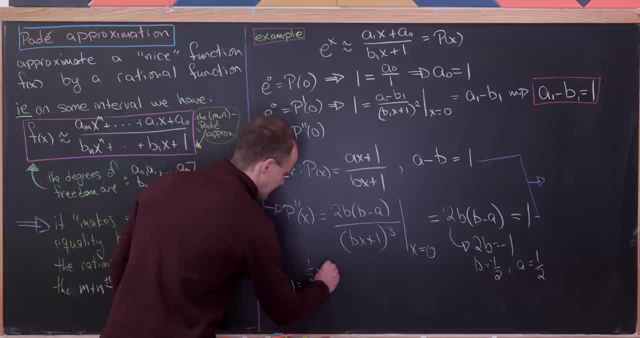 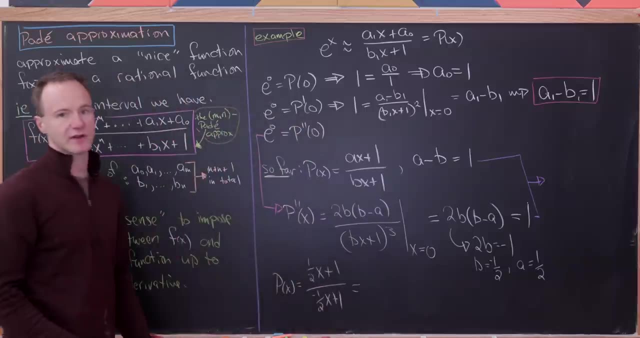 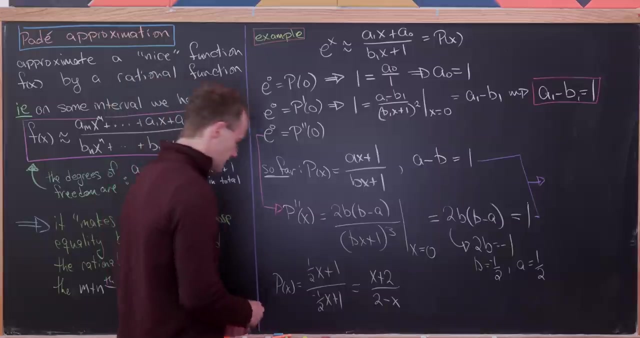 of x is now equal to a half x plus one over minus a half x plus one. Or we might as well multiply the numerator and the denominator by two to give us x plus two over two minus x. So let's maybe fit this in the upper corner over here we have our one comma, one pot, a approximate of e to the x, And this says that e to the x should be. 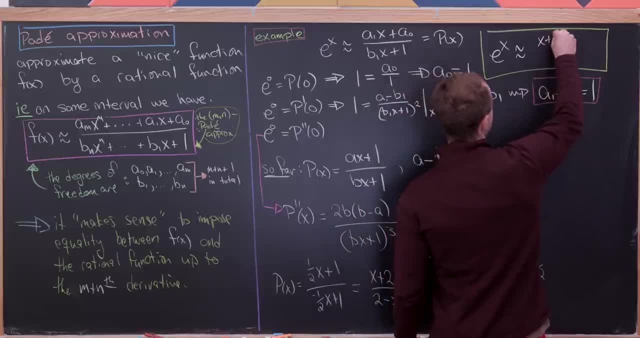 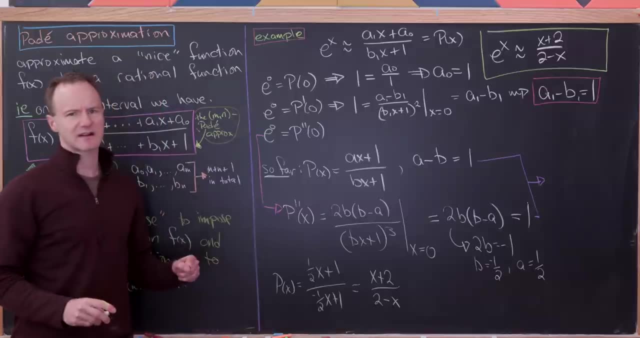 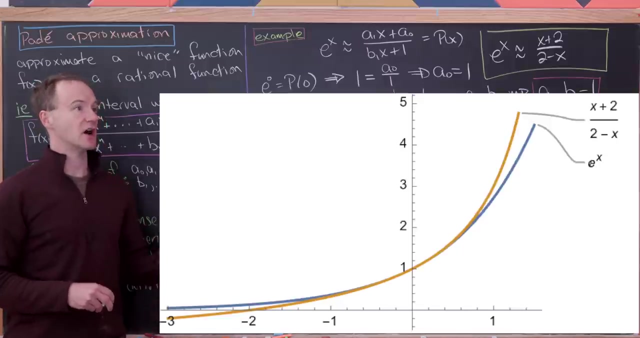 equal to n, approximately equal to x plus two over two minus x, on some interval containing zero, given the fact that we impose these conditions all at zero. Okay, so on the screen right now is a graph of these two functions and, as you can see, they're pretty close on that interval. Okay, let's do. 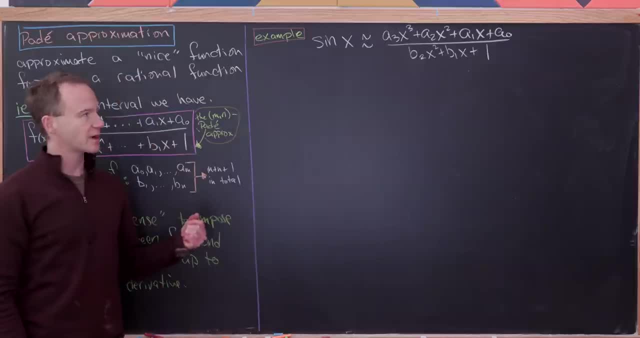 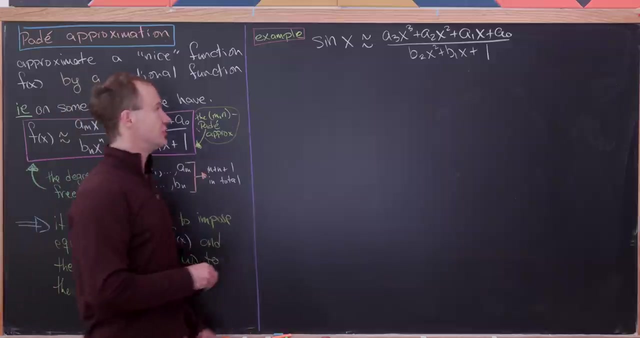 another example. Okay, so for our second example, where we're going to find the three comma two approximate of sine, we're going to use a different strategy, and this strategy is nice because it generalizes essentially to any nice function. So what we'll do is take sine and rewrite it. 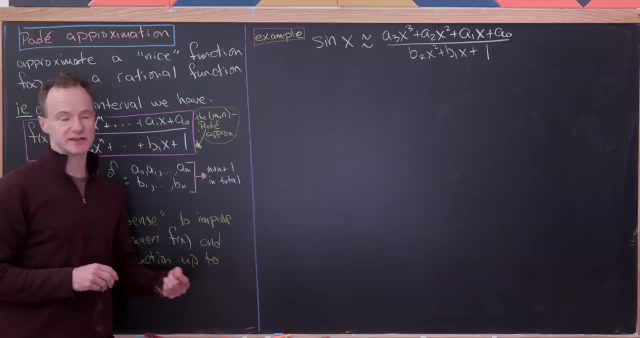 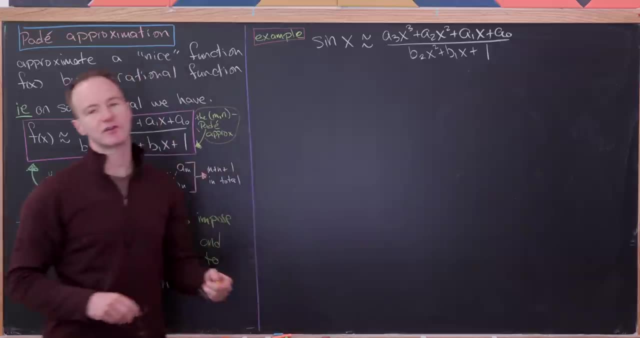 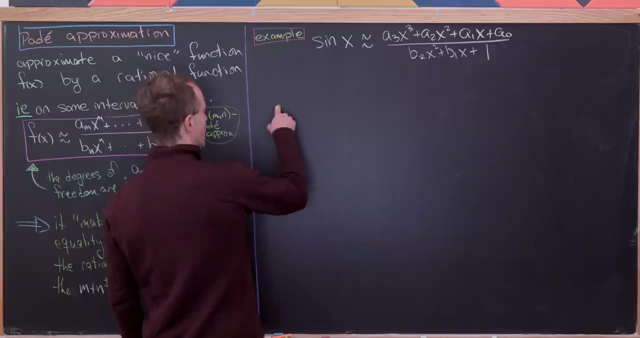 using its Taylor series. but we're going to truncate that Taylor series at a degree which is three Plus two, so the degree of the numerator plus the degree of the denominator. So let's see what that gives us. So what we should have here is x minus one over three, factorial x cubed and then plus. 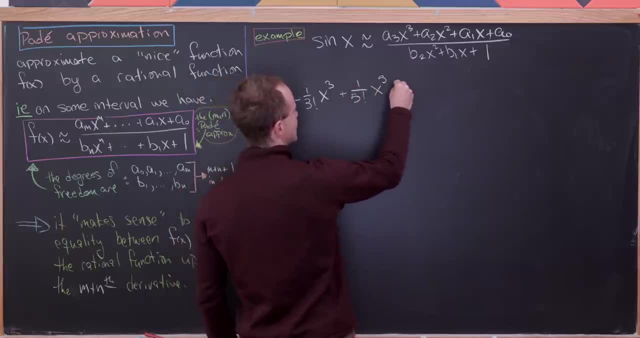 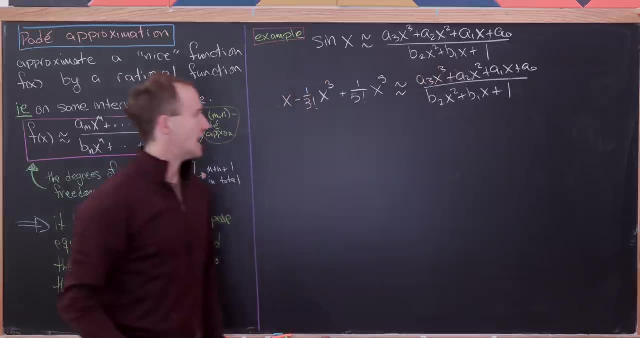 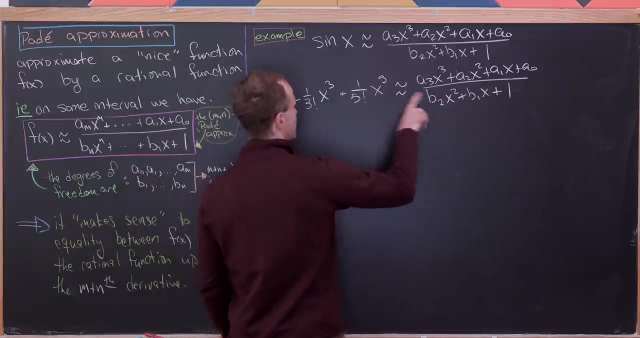 one over five factorial times x to the fifth should be approximately equal to our rational function, which I'll just recopy now And now. what we'll do is simply cross multiply. so we've got an equation of polynomials instead of an equation of a rational function on one side. So, in other words, I'm going to take the denominator up here and 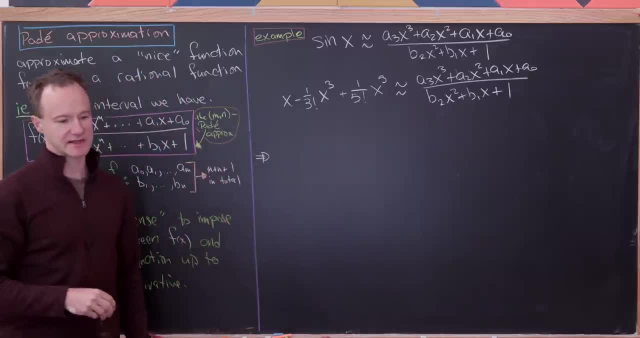 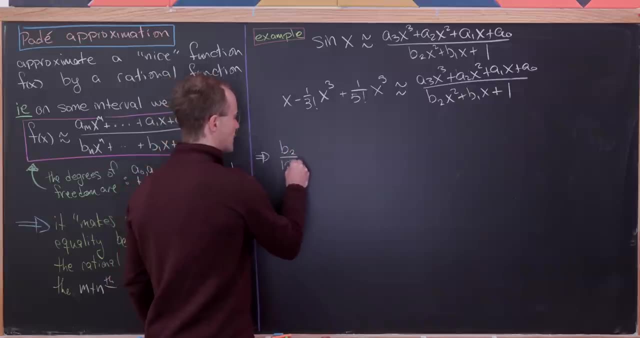 multiply it up to the numerator on the left hand side And that's going to give us the following object: So we'll have b2 over 120 times x to the seven. That's from the leading terms on both, And I'm going to get the rest of it copied over. Okay, so there we have it. We have it all written out. 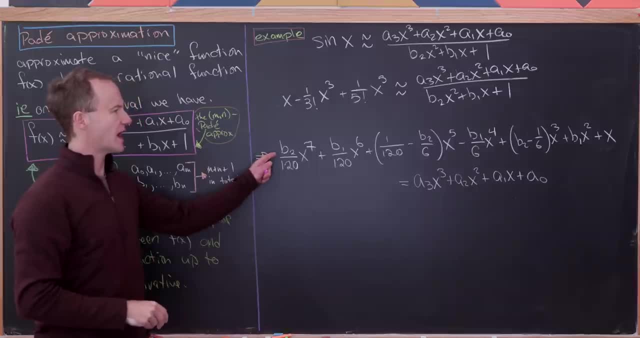 But what you'll notice is that there's no possible way to determine b2 and b1 using this setup. Or, in fact, maybe there's a way to do it, but it will contradict, but it will have contradictory equations Like: notice, the fact that we have no degree seven thing on the 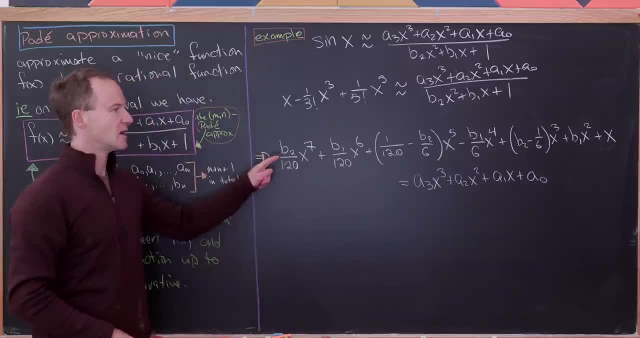 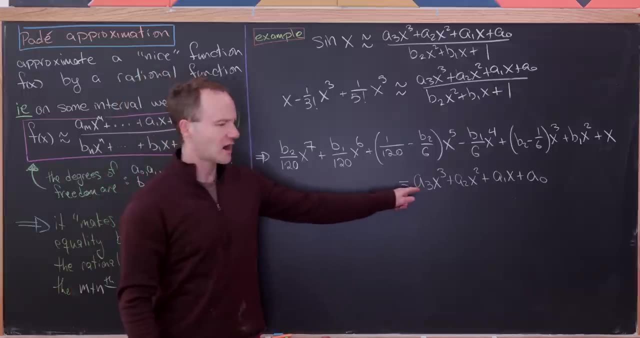 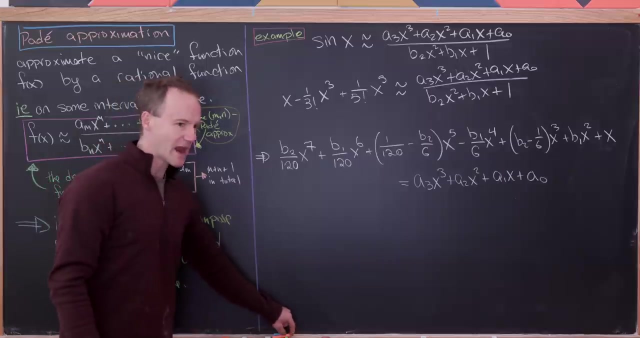 right hand side means that b2 has to be equal to zero. so that's what we want. So I'm going to take this zero, but then this b2 minus one sixth in the x cubed part, and then a- non a, possibly non-zero x cubed part here tells us that maybe b2 is not zero. so the way to do this is just to think that. 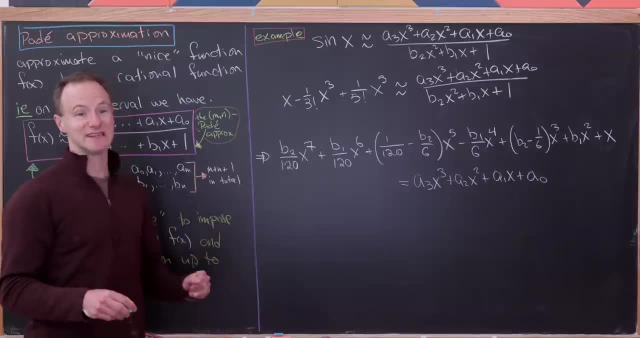 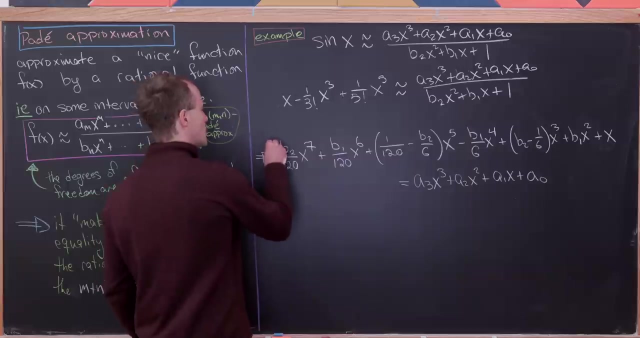 hey, we're approximating this very, very close to zero, and that's because we use the taylor polynomial of sine near zero. so that means x to the seven and x to the six are really small near zero, so we'll just kind of forget that these things are here. in other words, we're going to 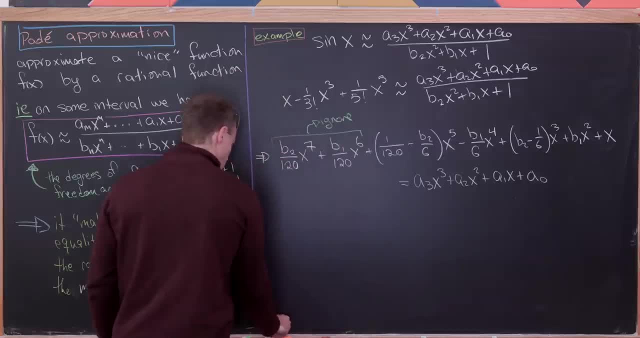 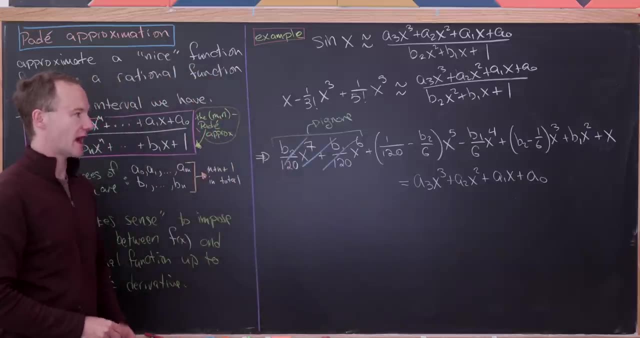 ignore these top terms. okay, great, so let's just get rid of these and then let's see the system of equations that's built from that. so observe that this x to the fifth term has got to be zero, because there's no x to the fifth on the. 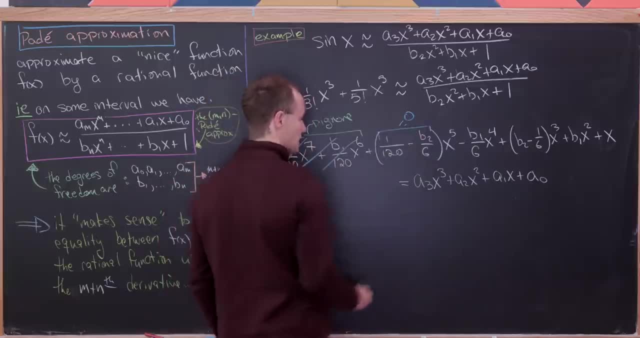 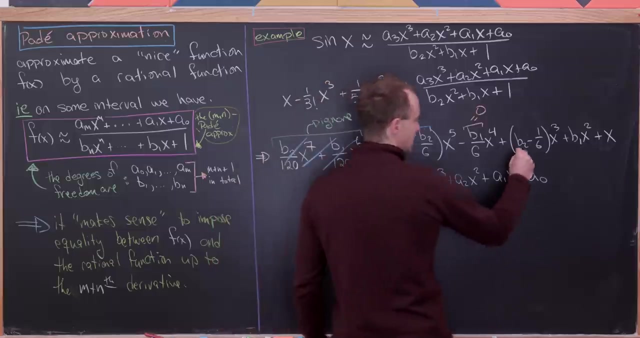 right hand side. so that gives us this must be equal to zero. then this x to the fourth term also needs to be equal to zero, because there's no x to the fourth term on the right hand side. and after that we'll need a sub three to be equal to b2 minus six, and then we'll need a. 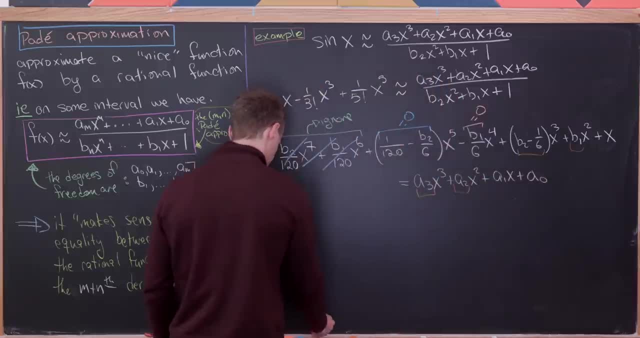 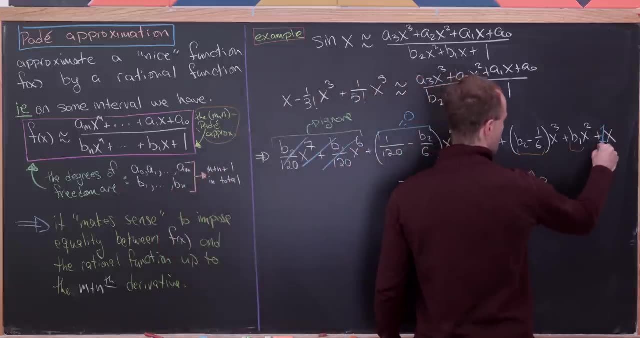 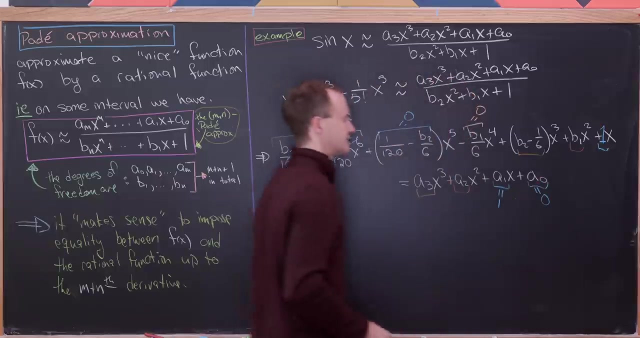 two to be equal to b one. because of those are the x squared terms, we'll need a one to be equal to. oh well, that just has a coefficient of 1, so that means that a1 is equal to 1 and then a0 must be equal to 0, because there's no constant term. 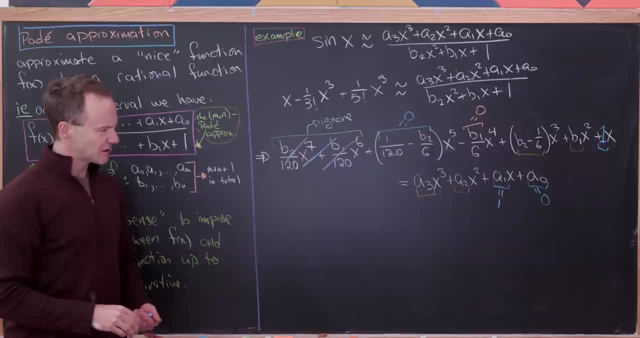 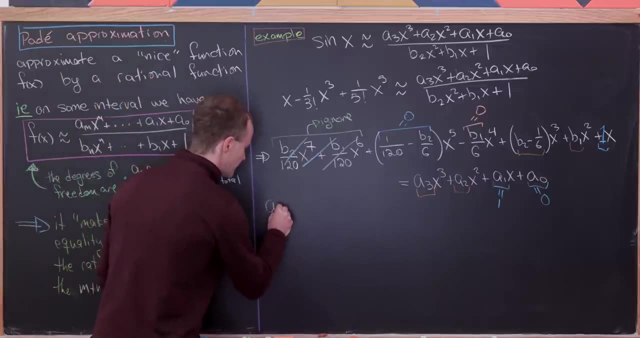 over there on the right hand side but observe that we're like getting values of our coefficients really quickly, so like let's collect those. so so far, we see that a0 is equal to 0, we see that a1 is equal to 1, and then, from this right, 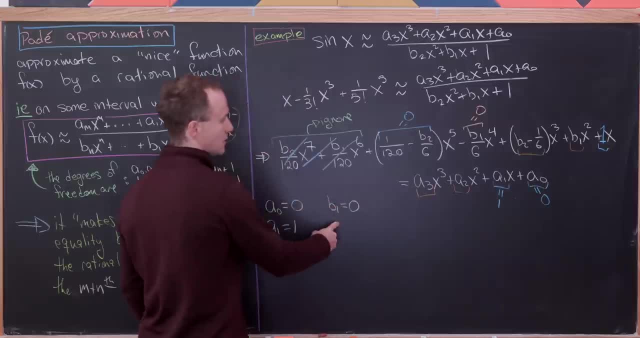 here we see that b1 is equal to 0. but then look at this: b1 and a2 are the same, so that means that a2 also is equal to 0. oh, but now let's look at this equation right here that involves b2. well, we can easily move some things around there and 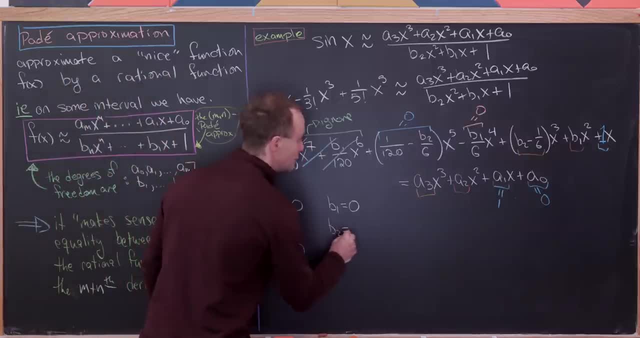 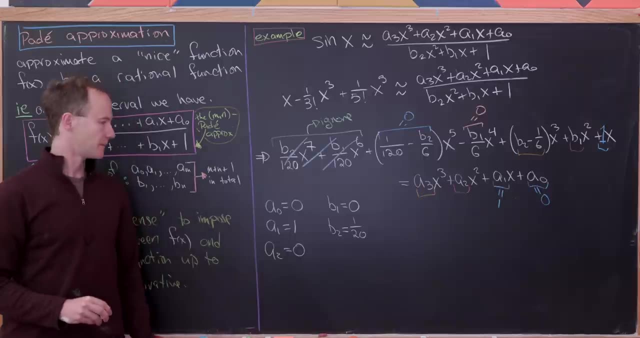 we'll get a value for b2, that is, b2 must be equal to 1 over 20. so that's a constant term over there on the right hand side and then from this. So that's just simple arithmetic. So that means we found the values of b1 and b2.. 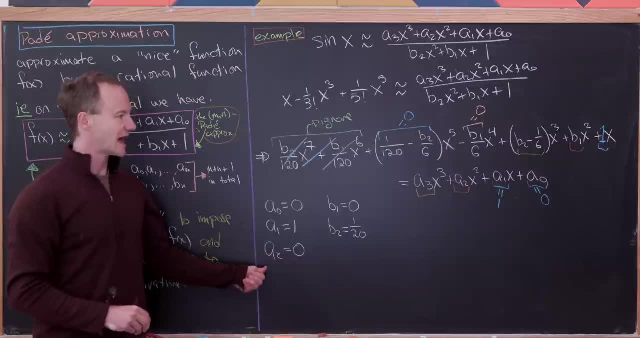 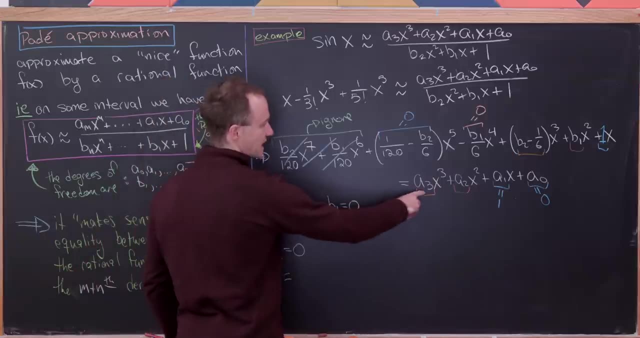 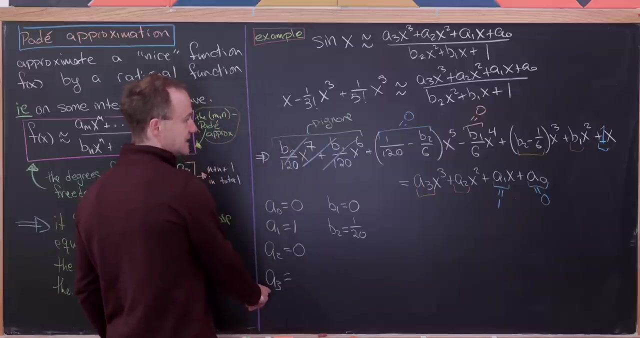 Those are the only values in the denominator that we needed, And the last thing we need to find is a3. But check it out. We know that a3 is equal to b2 minus 1 over 6.. So that means that a3 is equal to 1 over 20 minus 1 over 6.. 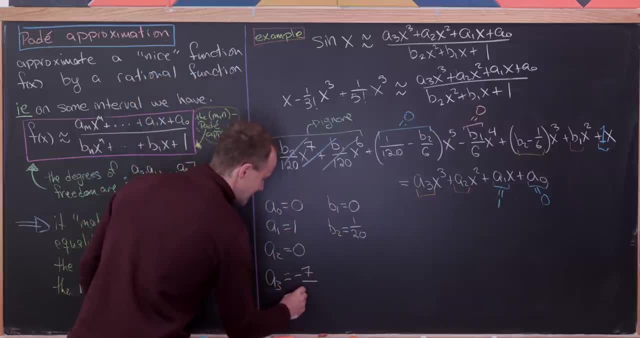 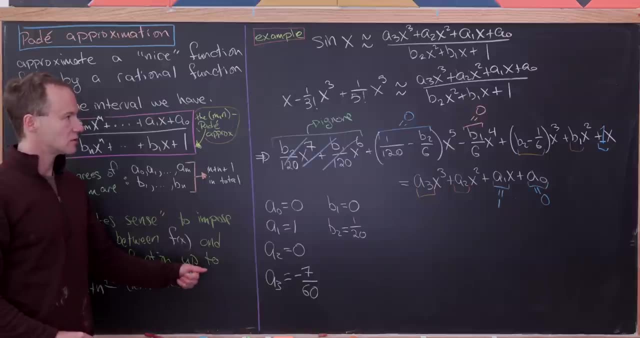 So you can do that calculation and you'll see that you get minus 7 over 60.. Okay, so those are all of our coefficients. So let's get those into our approximation up there And then, while we're at it, we'll clear denominators to make it look a little nicer. 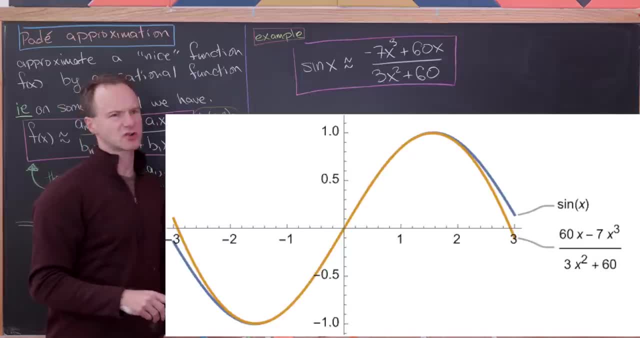 So there we have it. That's our 3-2 rational function approximation for sine. And again, I'll put an example of those plots on the screen right now so that you can see them. Okay, Now, how might this work in general? 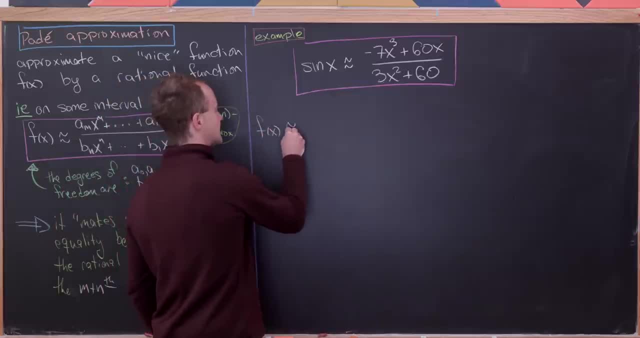 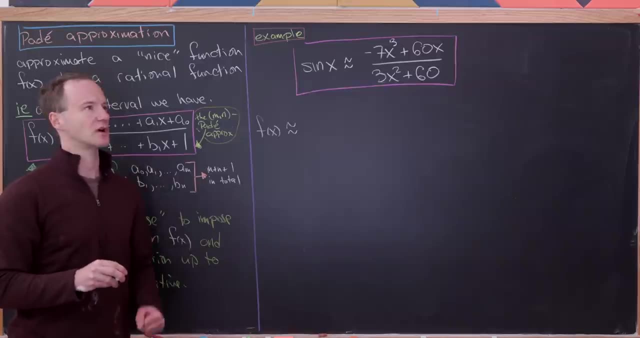 Well, let's say, generally you've got a function f of x And let's say you're allowed to take any derivatives of f of x. That is, it has a Taylor series approximation or a Taylor series expansion in some interval centered at 0.. 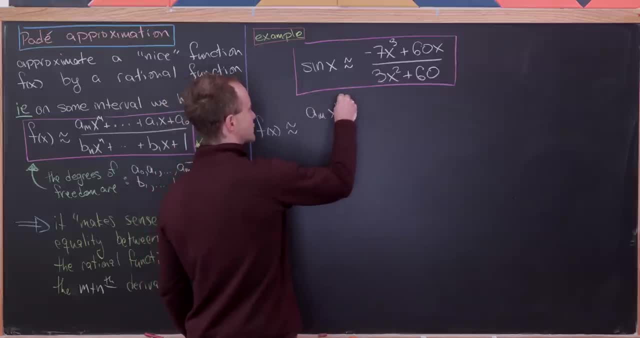 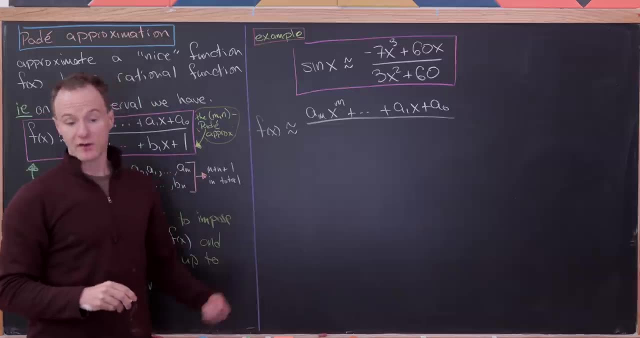 But we want to approximate it by one of these rational functions. So that means we want to approximate it with a quotient of a polynomial in the numerator, Like this, And then a polynomial in the denominator that takes this form that we've been working with. 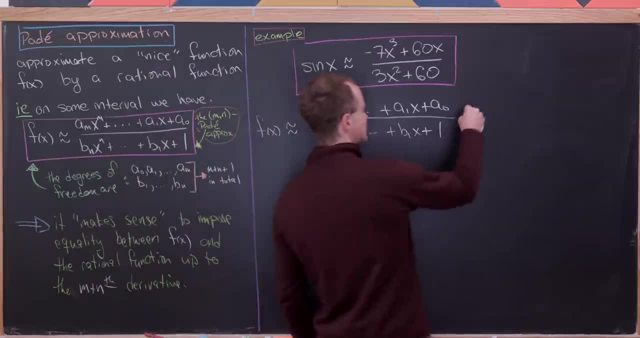 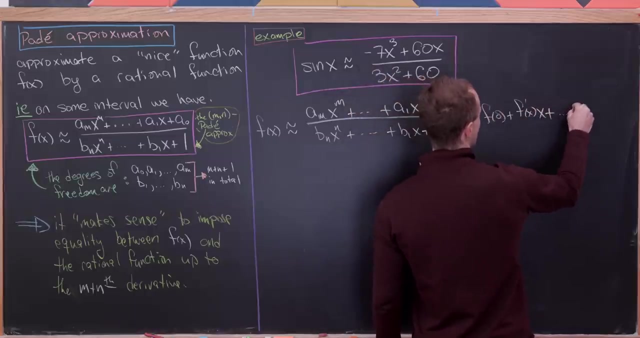 Okay, Great. And then, well, since we've got a Taylor series approximation, what we want is for this to be equal to, but it's not really equal to. it's approximately equal to f of 0 plus f, prime of 0 times x plus so on and so forth. 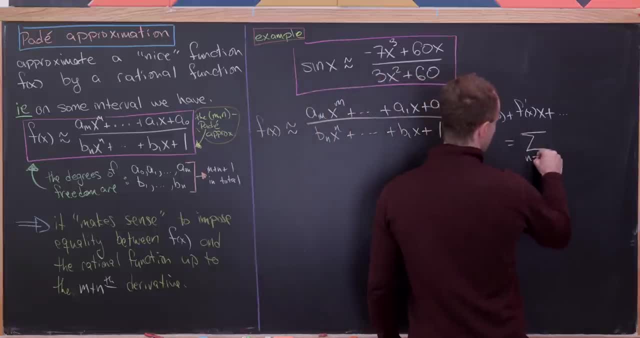 Or we could maybe write this out, Okay, Okay. Okay, The answer is the sum, as n goes from 0, or I shouldn't use n here. maybe k goes from 0 up to infinity of the kth derivative of f, evaluated at 0 over k factorial times x. 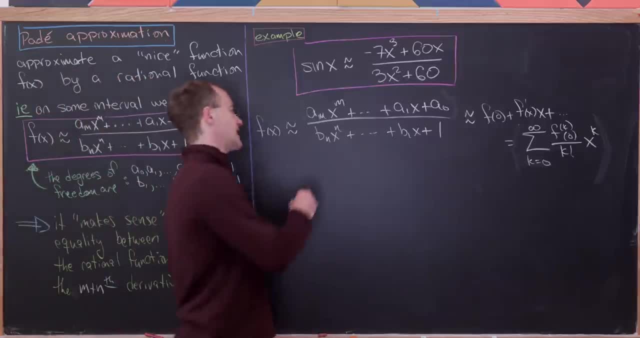 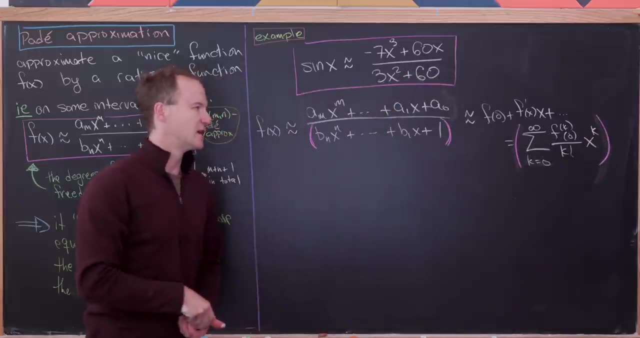 to the k And then next up. what we'll do is take the denominator over here on the left-hand side and then this numerator on the right-hand side and multiply them, giving us an equation of polynomials. You might say: well, I'm going to be left with n. 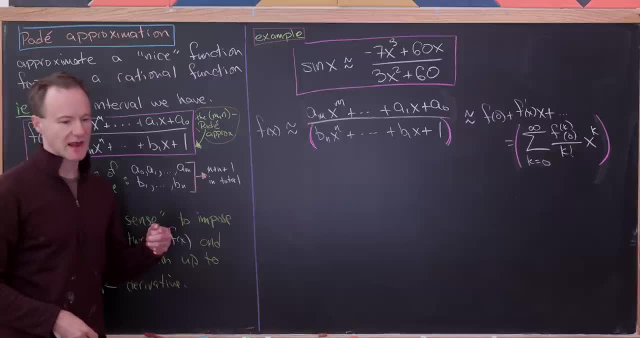 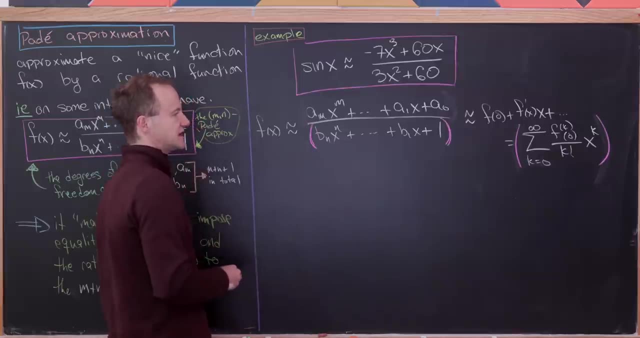 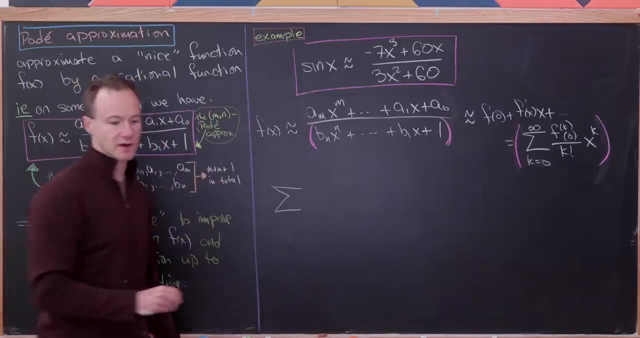 Okay, infinite series on one side, but we'll truncate that at x to the m plus n, much like we did in our example. So after multiplying those two things that have magenta parentheses, we'll have the following: and this is using the so-called Cauchy product formula for multiplying series, We'll have: 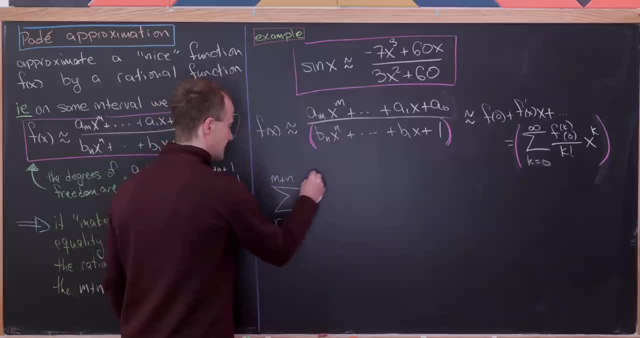 the sum as r goes from 0 to m plus n and inside of that we'll have the sum as s goes from 0 to r. We'll have the s derivative of f evaluated at 0 over s factorial and then b sub r minus x times. 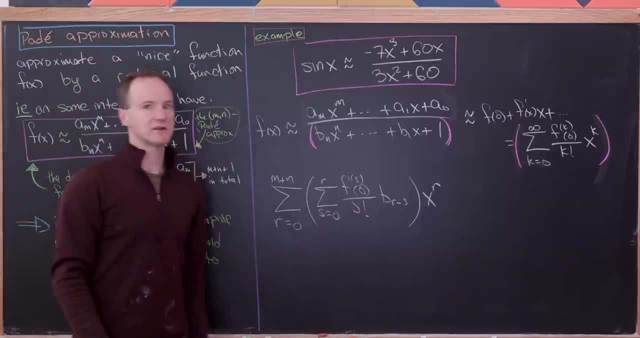 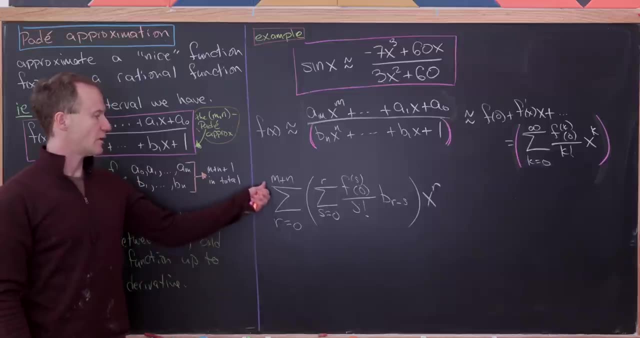 x to the r, And here, if you ever encounter a b sub 0, we'll take that to be equal to 1.. And then let's say, if we didn't truncate it, what we would have as a upper bound here of our sum would simply: 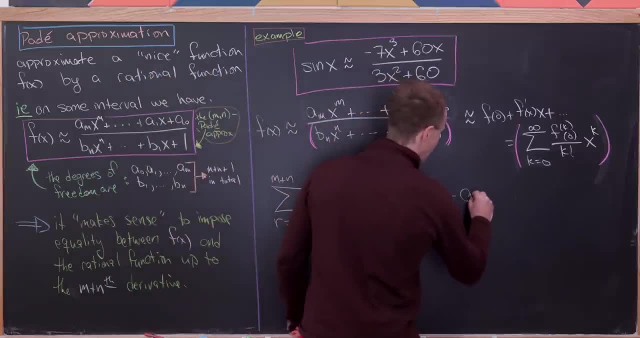 be infinity. And then over here we'll have a sub m x to the m added all the way down to a sub m x to the m, And then we'll have a sub m x to the m added all the way down to a sub m x to the m. 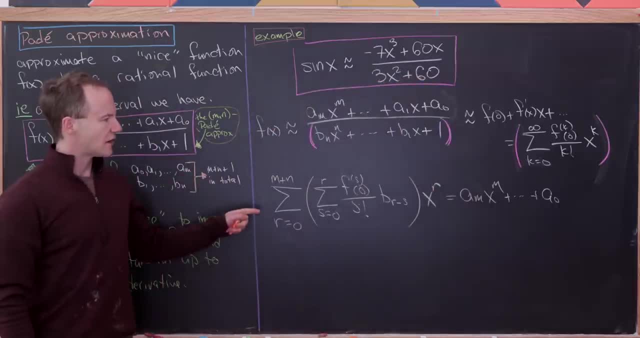 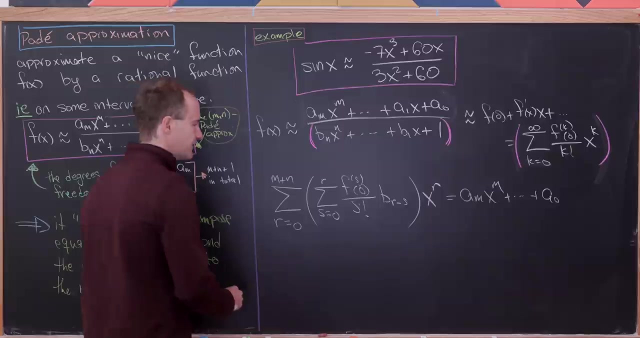 Sub 0. So now let's observe that we have more terms over here on the left than we have on the right. That means that when we build our system of equations, the top bunch of systems of equations are equal to 0. And in fact what we have is for r between m plus 1, so r between m plus 1 and m.